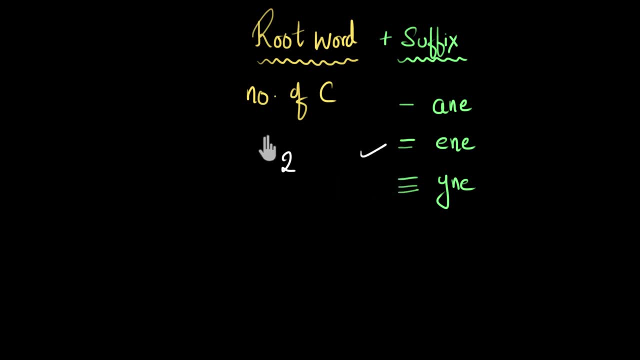 okay, and one double bond between them. With just these two information, you will be able to guess which hydrocarbon am I thinking of. You will write two carbons and then a double bond in between them. Rest, all valences will be satisfied. 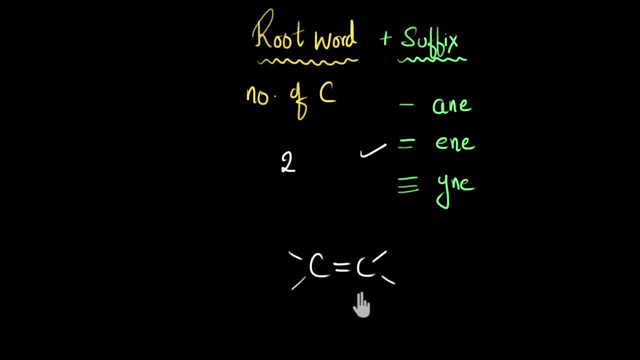 by hydrogen. That's why this is a hydrocarbon. So, yes, this is the hydrocarbon that I was thinking of. So, yes, these are the two information needed to name a hydrocarbon. Now let's look at each one of them in detail. So root words are words that denote the number of carbon atom present in the 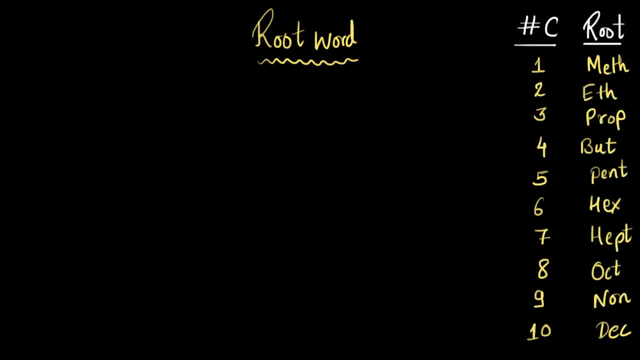 molecule, And traditionally we have been using these root words. If there is only one carbon atom, then we use the root word meth. For two, we use the word eth For three, prop For four, bute and so on and so forth. So for example, 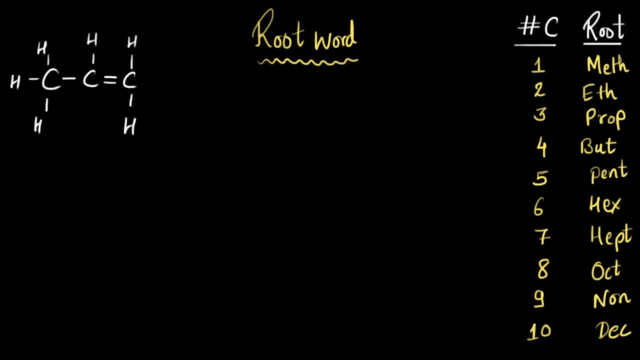 if I had this molecule to name. So first of all, I'll focus only on the carbon atoms. And here I see that there are three carbon atoms. So for three, to denote the presence of three carbon atoms, I will use the root word, prop. Let me write it down: Prop. Similarly, let's look at one more. 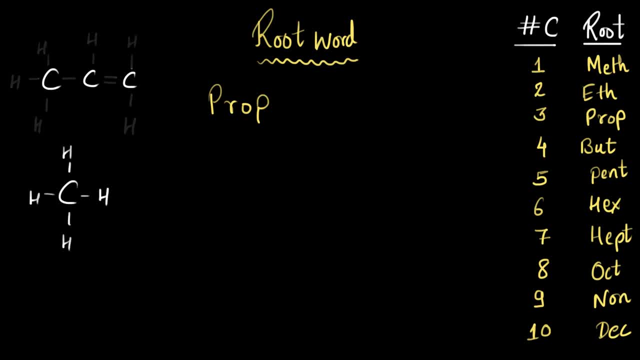 example, Let's try and guess what will be the root word for this compound. If you have tried it, let's see. See, this one has only one carbon atom, okay, And for one we use the root word meth. Let's look at one. 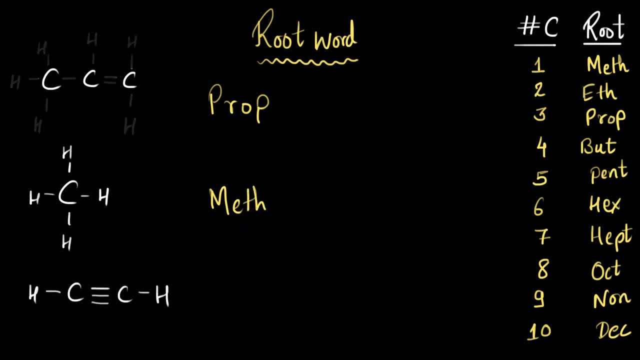 more example. Pause and try to name the root word for this one. So here, if you see, there are only two carbon atoms present. So here we will use the root word eth for this Eth. Now let's look at, Let's talk about the suffix. See, this is a word that gets added to the root word And it denotes: 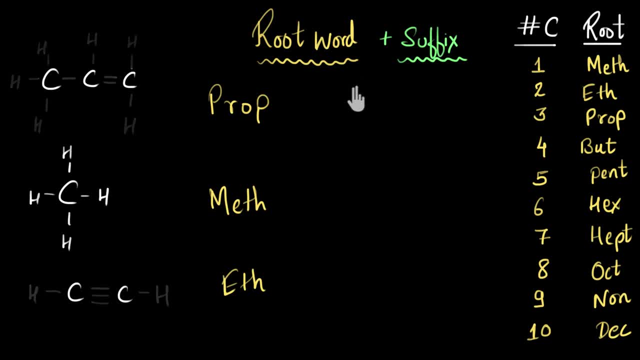 whether the molecule belongs to alkane, alkene or alkyne family. For example, if there are only single bonds between the carbon atoms, that means the molecule is an alkane and will have the suffix en added to the root word. If there is even one double bond between two carbon atoms, that means 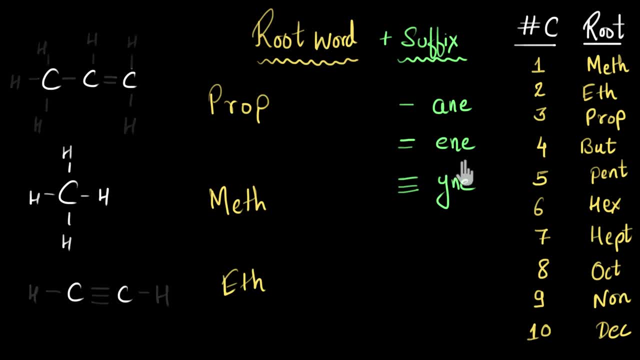 the molecule belongs to the alkene family and will have the suffix en added to the root word, And if there is even one triple bond that means the suffix will be ein, For example. let's look at the first molecule. So if I just focus on the bonds between 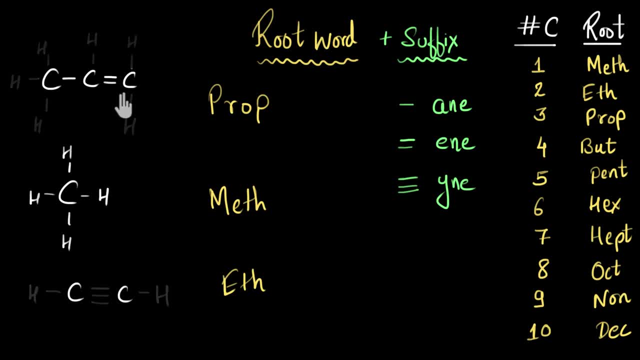 the carbon atoms, you can see that there is one double bond. Two carbon atoms have a double bond in between them. okay, So that means this carbon chain will belong to the alkene family And therefore the suffix added over here with the root word will be en. Let me write it down. 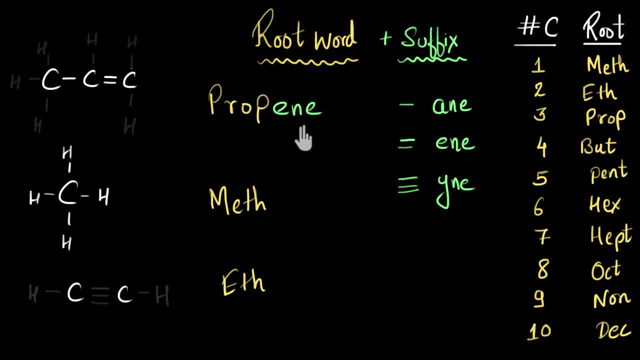 En, And so the name is going to be prop-en. Now, if you look at this example over here, you see that there is one carbon atom. okay, For alkane and alkene you need minimum two carbon atoms. So definitely this is an alkane, And for alkanes the suffix is en. So the suffix en. So. the name of this molecule will be methane. Now let's look at this example. If I just focus on the bonds between carbon atoms, you see that there is a triple bond between them, right? So that means this molecule belongs to the alkyne family and they will have the suffix en. So to the root. 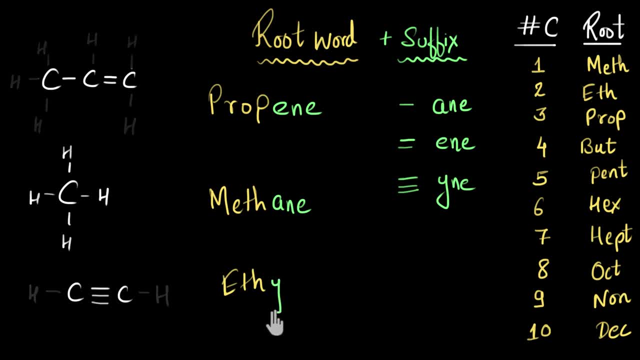 word we will add the suffix en, So the name of this molecule is going to be eth-en. So with this we saw how to name hydrocarbons Basically there are two parts: root word, which denotes the number of carbon atoms present, and suffix, which denotes whether it belongs to the alkane. 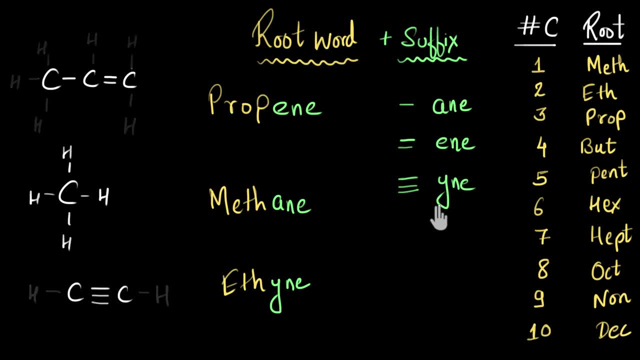 alkene or alkyne family. Now, one thing to note over here is that here we are only talking about single carbon chain molecules. okay, There is no branching. that is happening over here. When branching happens, the the rules of root word kind of changes a little bit. We'll talk about that in future videos. 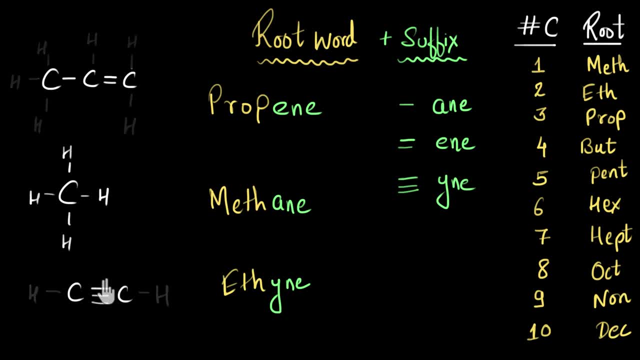 And also we are talking about simple alkenes and simple alkynes, meaning there are only going to be one double bond or one triple bond. There could be multiple double bonds in an alkene, okay, And for that the suffix rule kind of changes a little bit. We'll talk about that also in future. 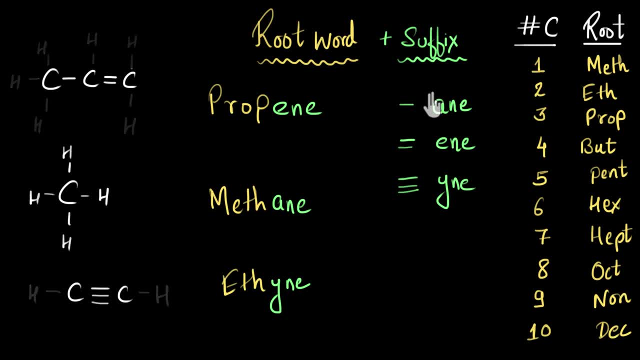 videos. Now, so far we have seen that if you are given the structure of a hydrocarbon, then how to write its name. Now, what if I give you the molecular formula of a hydrocarbon like C4H8? How will you write its name? Well, if you did not, 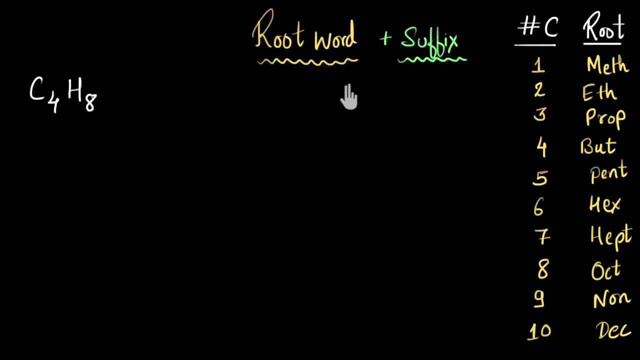 know anything, you would say that you know. I would go with the same logic. First I will find out the root word and then the suffix. So the root word denotes the number of carbon atoms, and that's easy to find out here. It's already given that there are four carbon atoms in this. 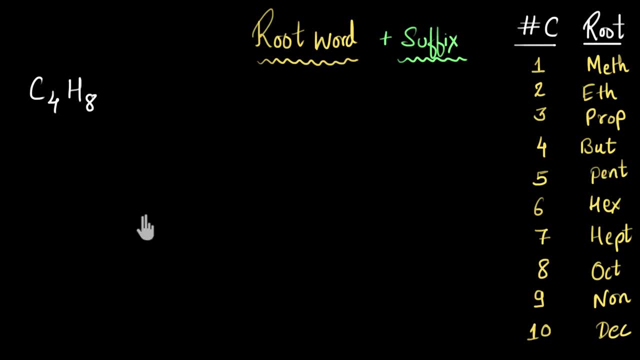 molecule. So for four we use the root word bute. So let me write that down. The root word for this molecule will be bute, Now suffix. This denotes whether the molecule belongs to the alkane family, alkene or alkyne family. 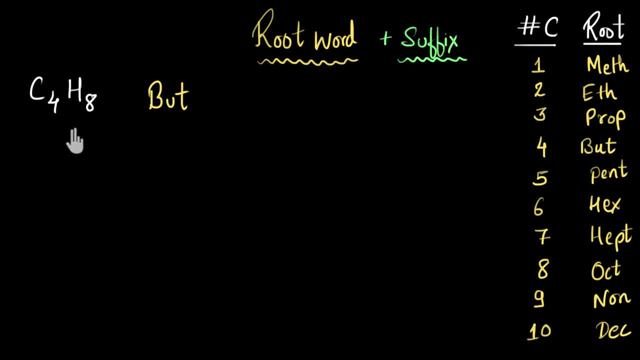 Now, how do we find that out? by just looking at the formula. Well, if you recall, in a previous video of alkane, alkene and alkynes, we talked about the general molecular formula. Alkanes general molecular formula was CnH2n plus two, which means that all the alkanes will have the 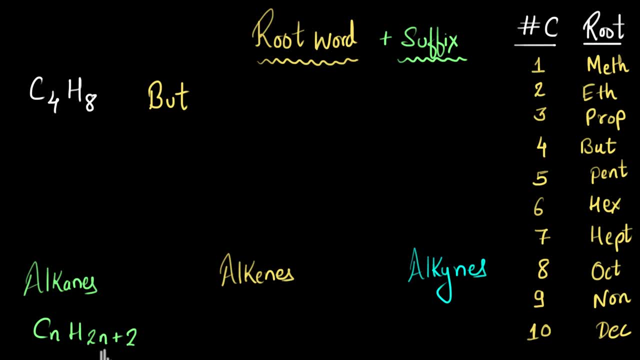 number of carbon atoms and hydrogen atoms in this proportion, Meaning all alkanes, their hydrogen atoms will be twice the number of hydrogen atoms than the carbon atoms. For alkynes, their general molecular formula was CnH2n minus two, meaning the hydrogen atoms will be twice carbon atoms minus two. okay, 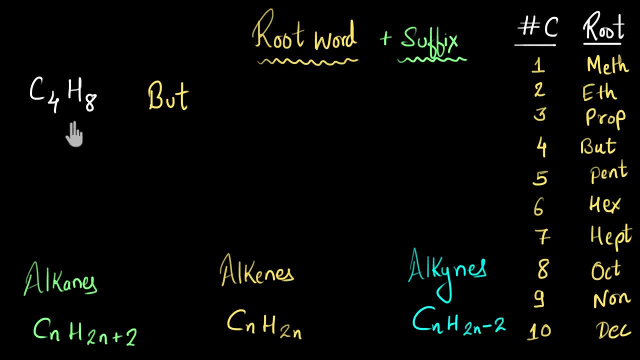 Now, using these, we will figure out whether this molecule is an alkane, alkene or an alkyne. So over here I can say that I have two carbon atoms, which means that the carbon atoms will be twice the number of carbon atoms and according to this formula, the hormone can be twice- twice the 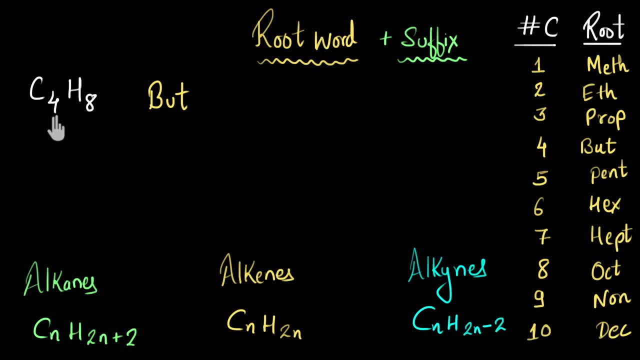 see that number of hydrogen atoms. this is twice the number of carbon atoms for two side right, and that only happens in the case of alkenes. Alkenes have twice the number of carbon atoms, so this should belong to the alkene family, and for alkene family the suffix used is: 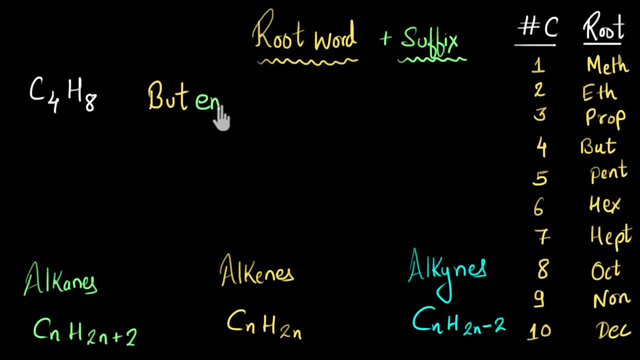 ene, So let me write that down: ene, So this molecule has to be butene. okay, Now, with this, let's see if we can solve a couple of more examples. Can you pause the video and try to find out their names? Now, if you have tried it, let's see. So this compound has six carbon atoms. 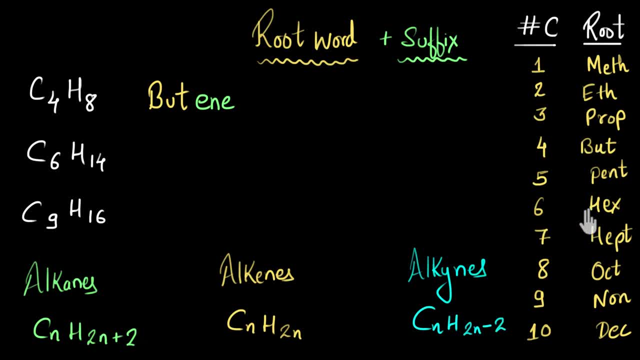 so for six, the root word used is hex. that will be the root word. Now let's talk about the suffix, whether this belongs to the alkene, alkene or alkene family. Well, how I like to remember is I quickly calculate whether the hydrogen number is twice that of carbon. If it is, then it will be.